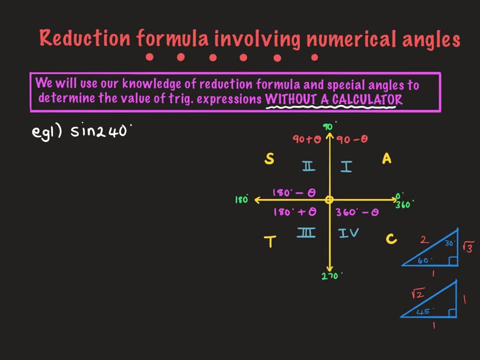 your calculator. now just check what you get If you type this into your calculator. your calculator says that this simplifies to negative root 3 over 2.. Okay, that's great, But if you just put that down as an answer in a test or exam, I would not be very impressed with you. You need to. 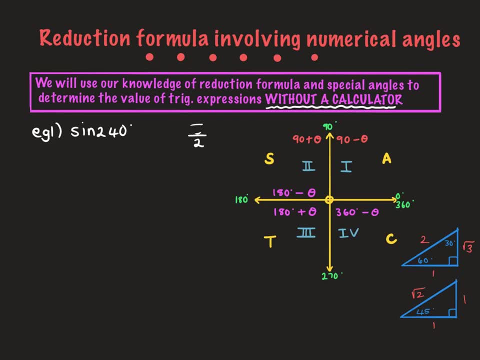 show your work. So let me show you how to show your work. It's pretty easy, guys. So this is the first thing I do: 240 degrees. Where is 240 degrees on the Cartesian plane? Right, You would agree, you should agree. it's in quadrant 3, right? It's between 180 and 270. 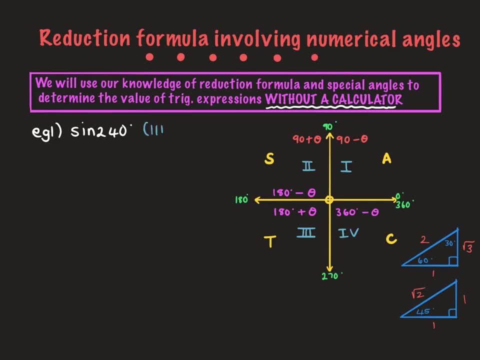 degrees. So that's the first thing I do. I identify my quadrant. I'm working in quadrant 3.. So I'm quadrant 3.. We know that quadrant 3 is the 180 plus theta quadrant. So grade 11s tell me. 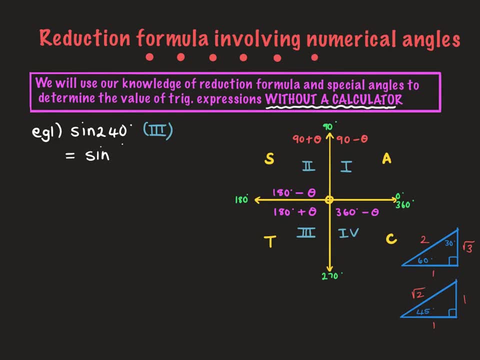 how can you rewrite 240 degrees as 180 plus something. So 180 plus 60 is the same as 240.. So 180 plus 60 degrees, this is equivalent, right? That says 240. That says 240.. So all you've done. 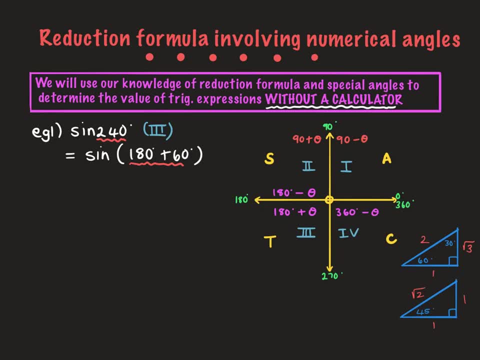 is. you've rewritten it as 180 plus an acute sized angle. The whole point of reduction formula is reducing down to an acute sized angle. So now we can go to our next step, which is when you are in quadrant 3, we know that this is where tan is positive, but sine and cos are. 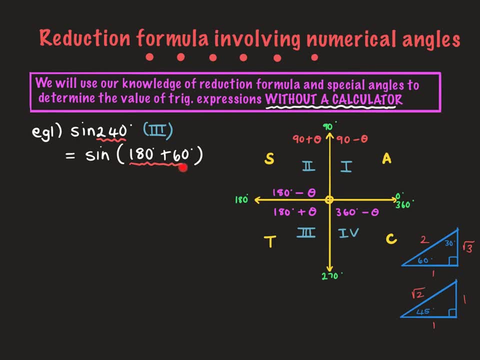 negative in quadrant 3, right. So now, when you apply your reduction formula here, so you're used to seeing 180 plus theta or 180 minus theta. Now, instead of theta, I actually have a numerical angle and I'm going to reduce down to that numerical angle, knowing that in quadrant 3,, 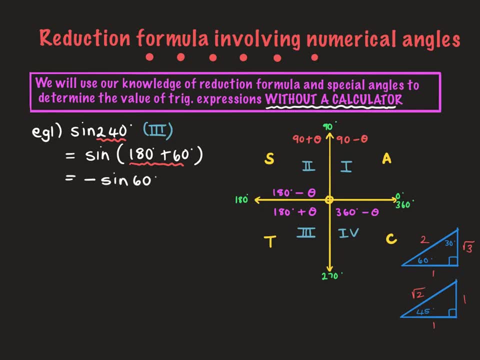 my function is negative, So I reduce down to negative sine of 60.. Now, using your special triangle, sine of 60 is opposite over hypotenuse. So my answer for this is negative root 3 over 2.. And right at the beginning of the question I said: if we just punch this into our calculator. 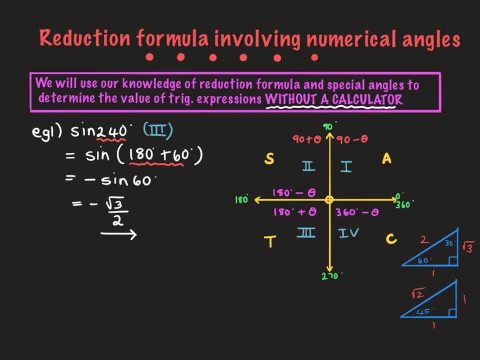 wasn't that the answer that the calculator gave us? Yes, it is. Isn't that easy peasy, lemon squeezy. So if I run through it again, you take the angle you've been given, identify your quadrants. That dictates: is it 180 plus 180 minus 360 minus? 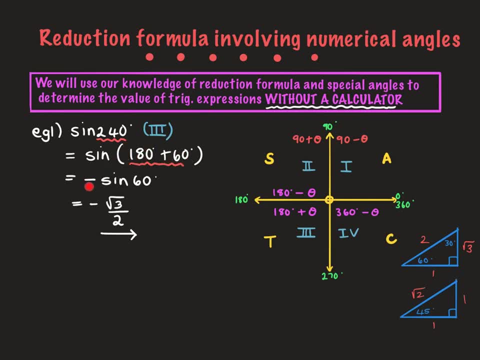 Then, whatever quadrant you're in, remember that your function will either be positive or negative. reduce down to that acute angle, use your special triangles. boom, there's your equation. That's your answer. Pretty flipping cool, I think at least. 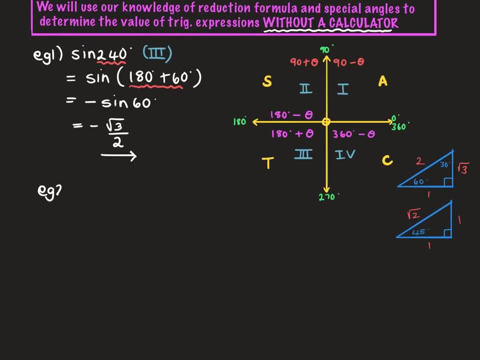 Okay, so let's try a second juicy example. How about I throw this at you: Cos of 330 degrees divided by fractions, tan of 135.. We don't let fractions bother us, right? Okay, so let me work through my steps. 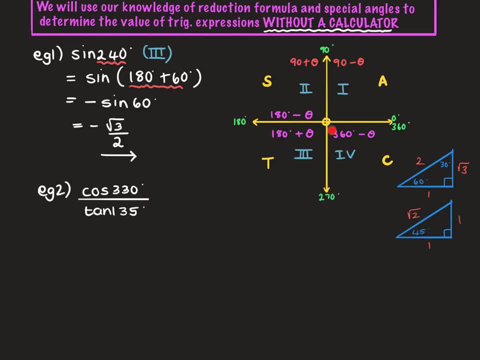 330 degrees, where you at 330 degrees is in quadrant 4.. Hey-ho, 135 degrees is in quadrant 2, between 90 and 180.. Awesome, So I've identified my quadrants: Quadrant 1, I mean quadrant 4 and quadrant 2.. 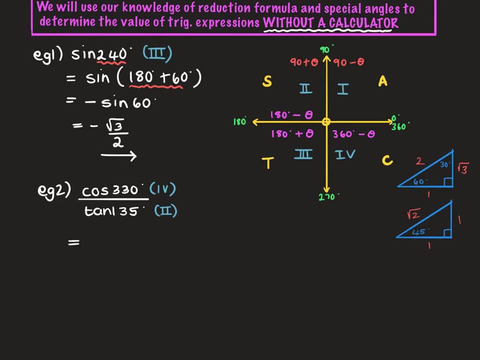 Lovely. So in quadrant 4, that's the 360 minus theta quadrant. So you ask yourself, grade 11s, 360 minus, what is going to take me to 330 degrees. So cos of 360 minus 30 is equivalent to 330 degrees, right? 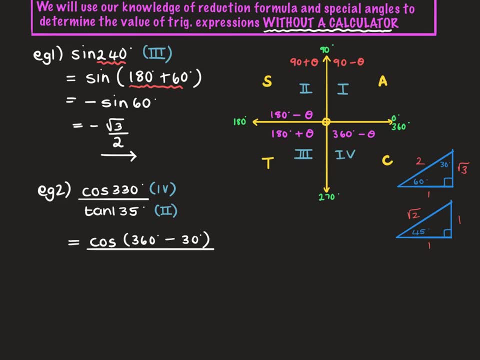 They're both saying the same thing. How about tan 135?? Well, in quadrant 2, that's the 180 minus 30.. Well, in quadrant 2, that's the 180 minus 30.. That's the theta quadrant. 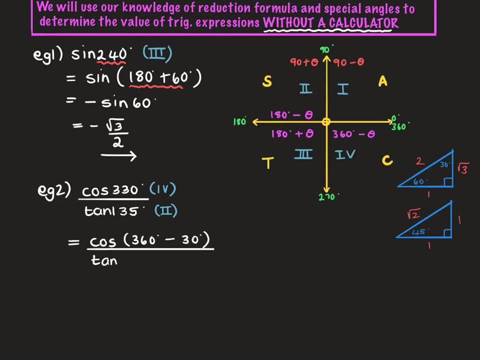 So 180 minus what is 135?? And you should be going: it's 180 minus 45 degrees clear. And I'm going: yes, you genius, Yes, you're right. Well done, So now what's the next step? 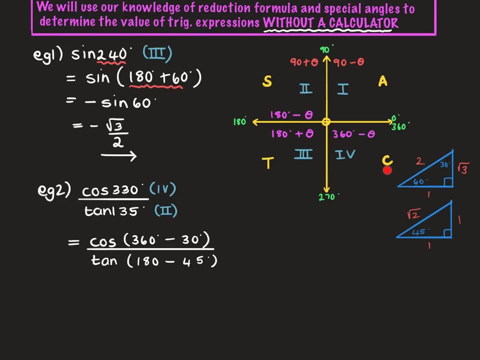 Okay. in quadrant 4, is cos positive or negative? It's positive, Okay, So it's going to pop out as positive cos. Now reduce down to the acute angle So that just becomes positive. cos 30 divided by right. in quadrant 2,: is tan positive or negative? 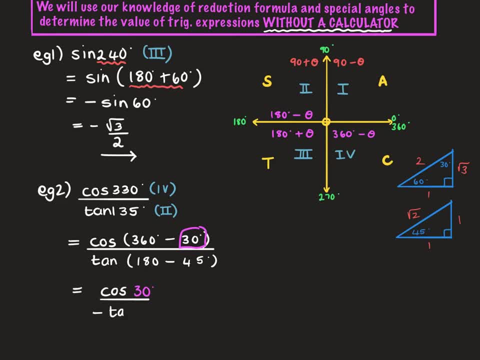 We know it's negative, right, So it's negative tan. And then what do you do? Reduce down to the acute angle So that becomes negative tan. 45. Pretty easy. So now that we've got these little juicy numbers, we go to our special triangles and I go. so cos of 30 is equivalent to sine of 60,, by the way, because of co-functions. 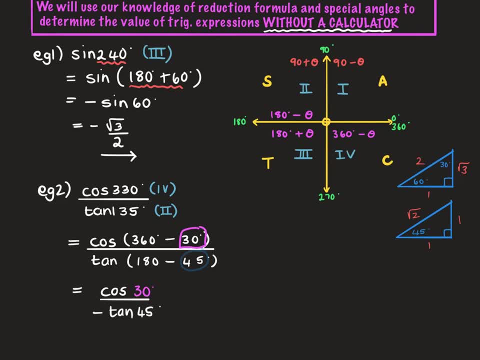 Yes, So cos of 30 is also root 3 over 2.. So cos of 30, root 3 over 2, divided by. so I'm saying the same thing right If I use a divide sign or that line: negative tan 45.. 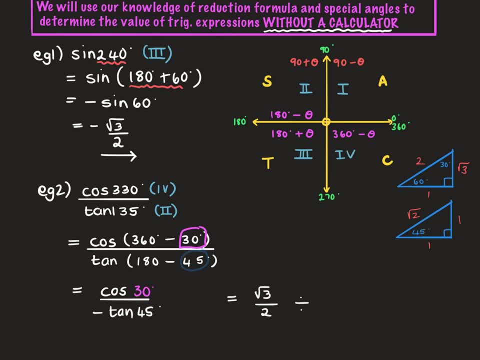 So tan is opposite over adjacent, So negative 1 over 1 or just negative 1.. So anything divided by negative 1 would just stay itself, But this will become negative root 3 over 2.. Hey-ho presto, you've answered the question and you are amazing. Well done. So in my next example, I'm going to use the root 3 over 2.. So in my next example, I'm going to use the root 3 over 2.. So in my next example, I'm going to use the root 3 over 2.. 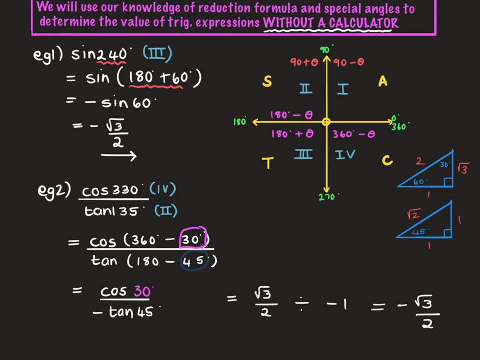 So in my next example, I'm going to go from step 1 straight to this step over here, This step in the middle. it's not really necessary to show this step And the more we practice this, you are not going to, you're not going to need to rely on this step anymore. grade 11s. 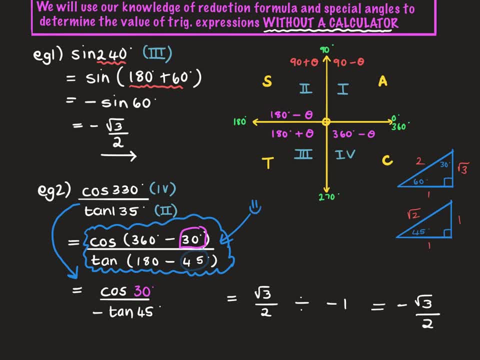 It's just for now, while we're really getting the hang of it. Okay, But in my third example I'm going to talk through the second step And we're just going to jump to our third step. So let me show you how we do this. 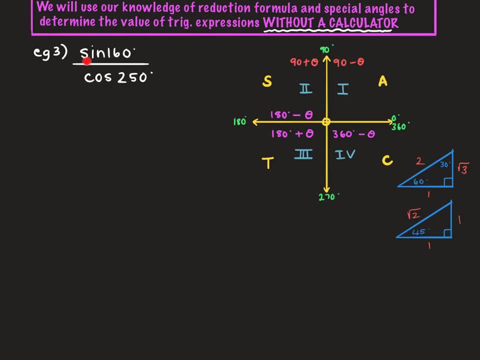 Cool. So let's have a look at our third example. All right, Sine of 160 divided by cos 250.. Cool, So 160 degrees. which quadrant am I in? I'm in quadrant 2.. Okay, So for now I'm still going to do this to help us. 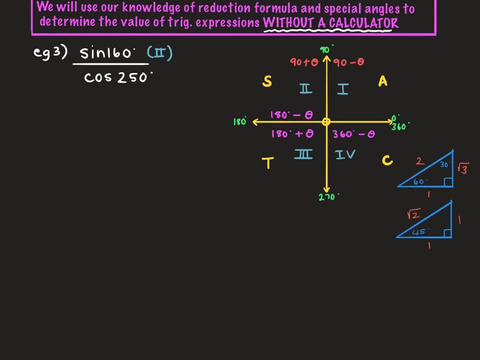 I'm in quadrant 2 with 160 degrees, And 250 would be in quadrant 3, right Between Between 180 and 270.. So I'm working in quadrant 1 and in quadrant 3.. Okay, So, like I said, we're just going to jump now. 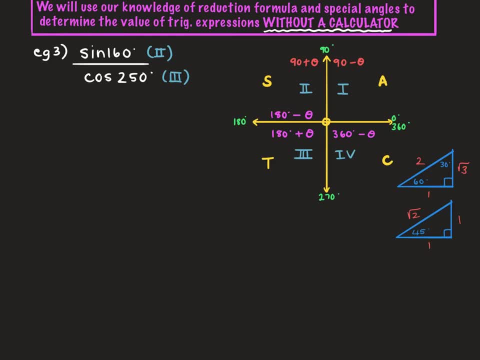 We're going to jump to that third step. I'm not going to do the step in between. So 180 minus what is the same as sine 160?? Well, sine of 180 minus 20 would take me to 160. So look at. 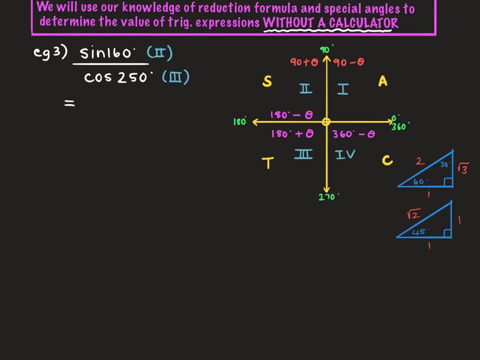 Grade 11s. I'm going to do everything in one step. I'm in quadrant 2.. So sine is positive in quadrant 2.. 180 minus 20 is the same as 160.. Okay, So I just did that in one step. 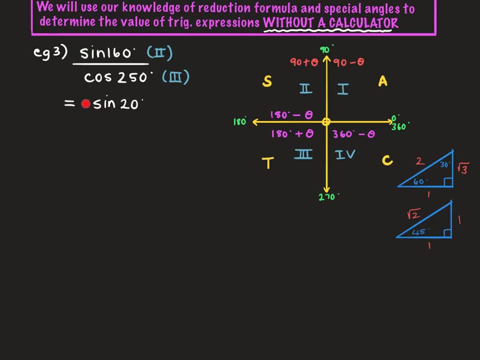 And we know now that these are equivalent. They have the same value. This is just the reduced down value of sine 160.. If you really like putting that middle step down, you are welcome to. All right, You don't have to do it this way. 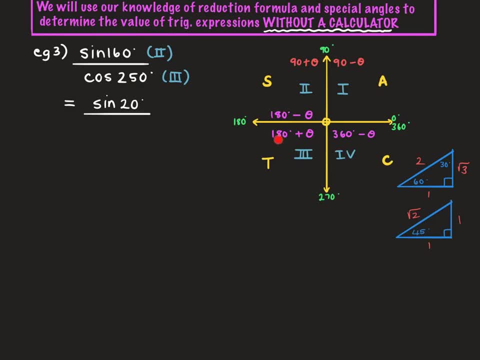 Cos 250.. Okay, So that's the 180 plus quadrant. So 180 plus what is the same as 250? Right, 180 plus 70.. So in quadrant 3, cos is negative. We just said we're going to go 180 plus 70.. 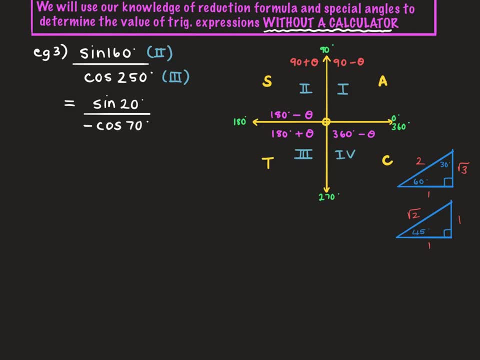 And we reduce down, Okay, To the acute size angle, Okay, So this is now what we left to simplify. And now you're going- oh goodness gracious Claire, 20,, 70. These are my special angles And I'd go. you are 100% correct. 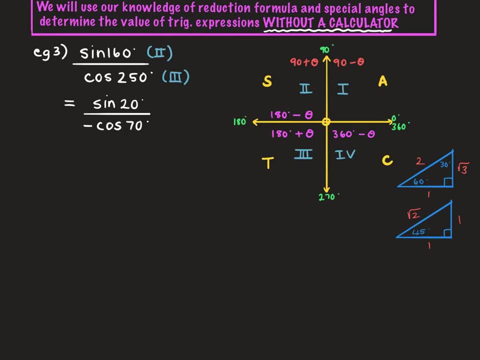 So how can I simplify this further? Something should be jumping out at you. Look at these angles: 20 and 70. What do 20 and 70 add up to? They add up to 90 degrees. So we know that when I'm working with sine and cos. 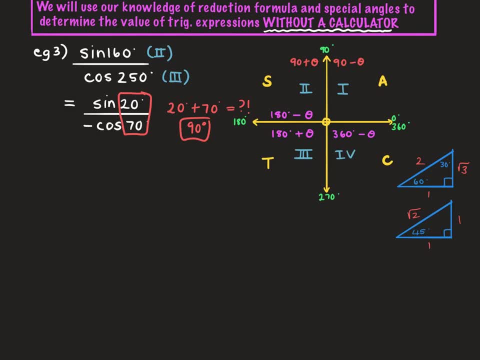 when the angles add up to 90,. this is when we use co-functions. Amazing right. So you can decide which. if you want to switch the numerator or the denominator, I'm going to leave sine of 20 as it is in the numerator. 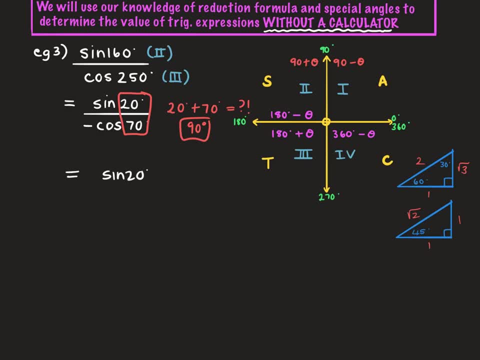 Now cos 70.. Cos 70. So that's in quadrant One right between zero and 90. So I can rewrite cos 70 as cos 90 minus 20.. All right, Cos 90 minus 20.. Let me write it here. 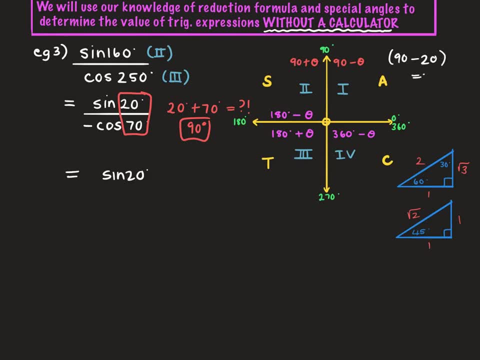 So 90 minus 20.. We know that that is 70 degrees And we know that in quadrant one all your functions are positive. So when it switches to sine it would switch to positive Sine 20. Remember, we reduce down to the acute angle. 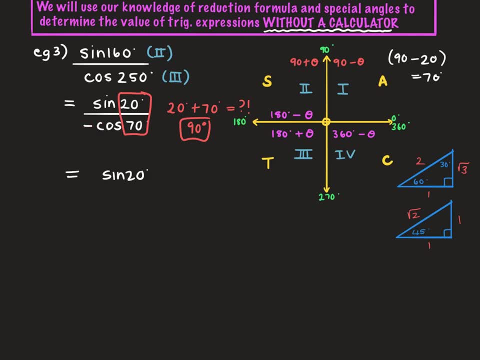 So it switches to positive sine 20, but it was negative to start off with And we know that a plus and a minus makes it a minus. So cos of 70 is the same as sine of 20.. So negative cos 70 is equivalent to negative sine 20.. 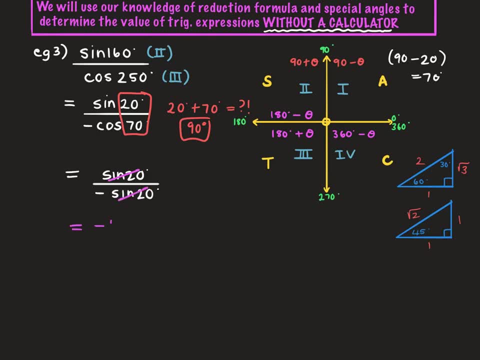 Now these are exactly the same And I get a nice juicy easy answer of minus one. And again, if you wanted to go punch it into your calculator, your calculator should say this: simplifies to minus one. Aren't these questions actually quite fun? 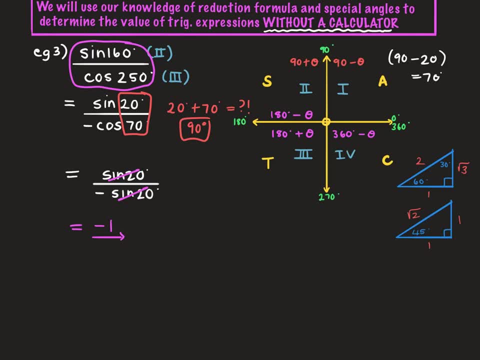 I really enjoy it. Let's try one more example: Okie dokes. Let's have a look at our last example, And I need to chat a little bit about these negative angles over here, So let's just deal with this first. 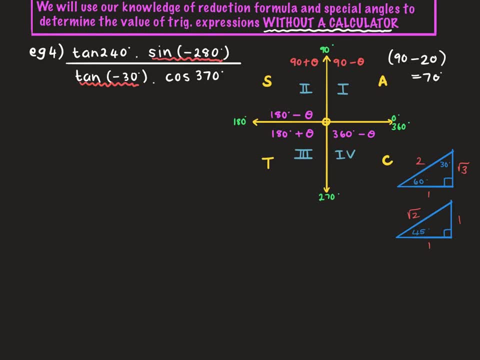 Before we start Identifying quadrants and reducing down to acute angles, Let's just talk about these negative angles first. So, negative angles. We're dealing with quadrant four then right. So I haven't drawn it on our cost diagram, but this is the negative theta quadrant, right. 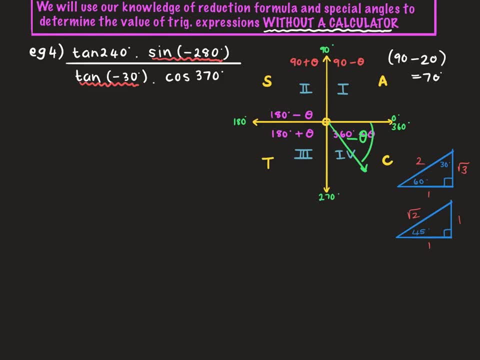 It's in quadrant four And we know that quadrant four is where cos is positive. So when we just remind ourselves four the negative angles for sine of negative, of a negative angle, So for instance, sine of negative theta, that would come out as negative sine theta for cos. 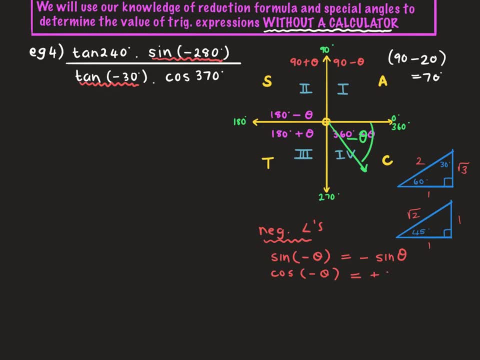 Remember that we've moved into its quadrant. So cos is the only one that pops out as a positive when we simplify the negative angle. But for tan, tan is the same as sine right. We're working in quadrant four. That's where 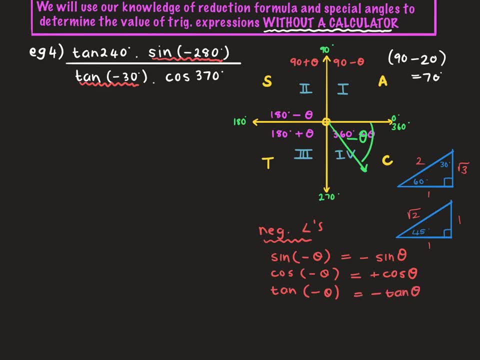 tan is negative, Sine is negative but cos is positive. So tan of negative theta would be negative tan theta. So we're going to deal with those negative angles first before I start reducing down. So tan of 240, I'm just going to leave it for now. 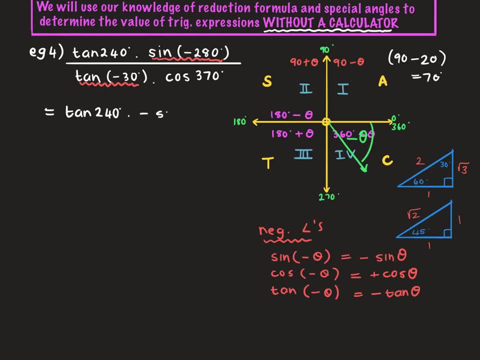 So sine of a negative angle becomes negative sine and the angle, which in this case is 280.. Right in our denominator, So tan of negative 30,, thinking of our negative angles, that will become negative tan 30 degrees Now, cos of 370. 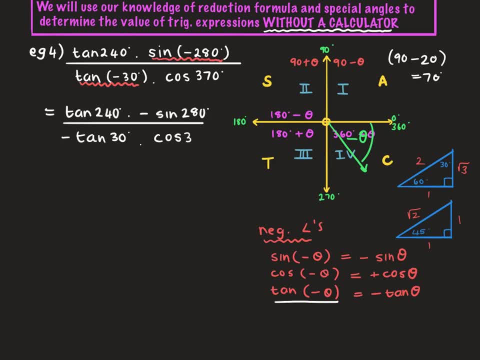 That's interesting Because 370 degrees- if we think about our cos diagram right, which runs from 0 to 360, 370 degrees would mean we're starting. we're starting a new revolution, So we're actually working again in quadrant one. 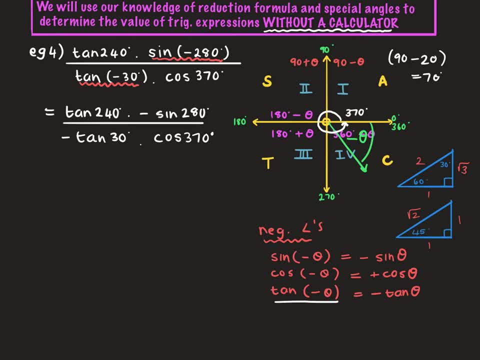 So I'm going to teach you a very handy trick. When you have angles which are bigger than 360 degrees, all you're going to do is subtract 360 from the given angle, And you're going to subtract until you have an angle which lies from 0 to 360. 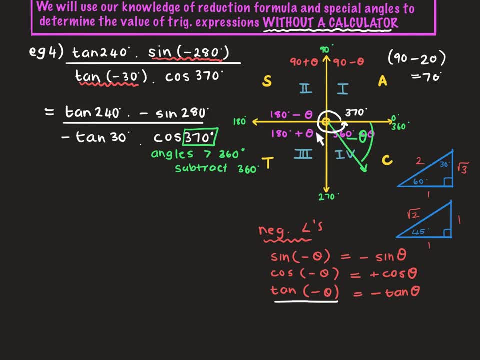 Because basically you want to be on your this cos diagram right working with angles between 0 and 360. So if your angles are bigger than 360, subtract until your angle lies in this range. But you can clearly see as well. 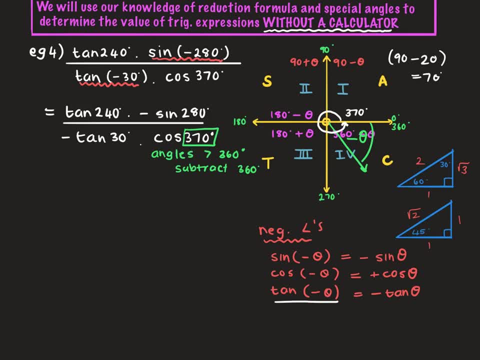 we're in quadrant one, So we know that this will come out as positive. So let me just show you that step. So I'm doing quite a few steps here. We can do it more quickly, more efficiently. but just for clarity. 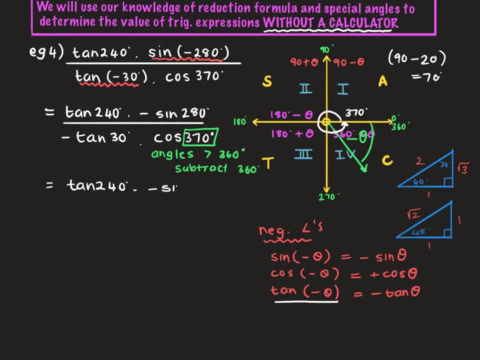 I'm going to show you what I mean. All right, So this for now, we're just going to leave as is. We're just going to deal with that angle bigger than 360.. All right, So we have our negative 10,. 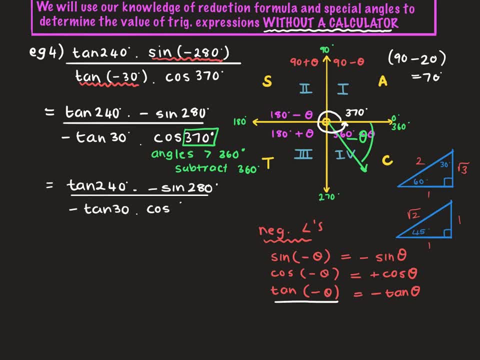 30 times. Okay, So you go cos. then you take your angle that's bigger than 360 and you subtract 360 degrees And that will simplify to cos of 10 degrees. Do you agree with me? 370 minus 360 is cos of 10.. 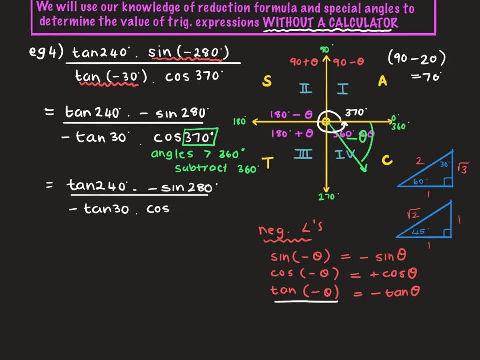 So I've shown you what that step would be. I'm just going to give you a simplified version. So that would be cos of 10 degrees, Cool. So now we can actually get to simplifying this down to a numerical answer. All right, 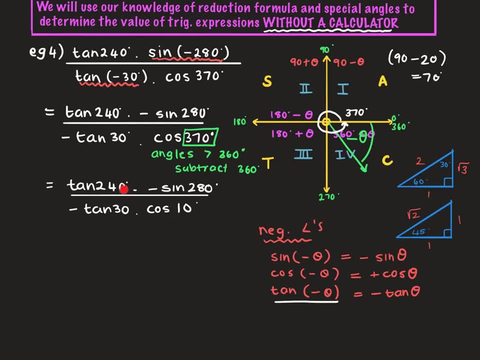 So let's go through this. 240 degrees lies in quadrant three, Where tan is positive. So I know this will be positive tan And then I say it's the 180 plus theta quadrant. So 180 plus 60 would take me to 240 degrees times. 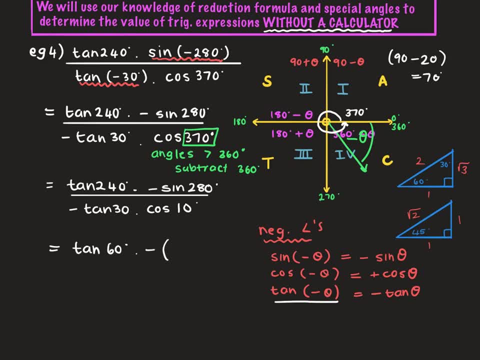 All right, Negative. So that negative is there. from working with the negative angle, which we know, since we're in quadrant four, sine will come out as a negative. Now I'm going to deal with sine 280.. Okay, So 280 degrees would lie in quadrant four. 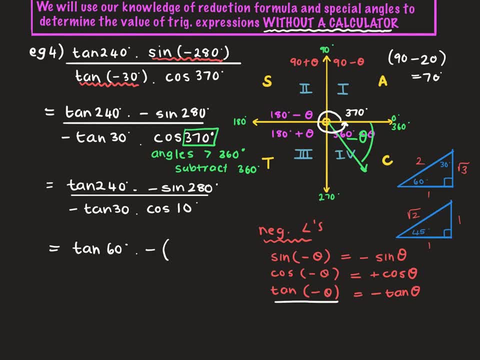 So we know that in quadrant four our sine function is negative, So it's negative sine. Now, 360 minus 80 will take me to sine of 280.. So that simplifies to negative sine 80. And we can see. 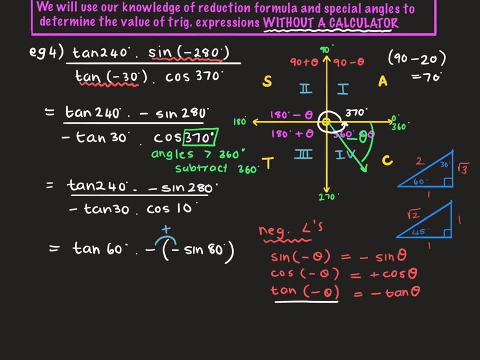 here that we know that that will become a positive. If you wanted to, at this step we could have also used our co functions idea And from 270 degrees we could have said sine 280 or 270 plus 10. And then we could have straight away switched to cos using our co functions. 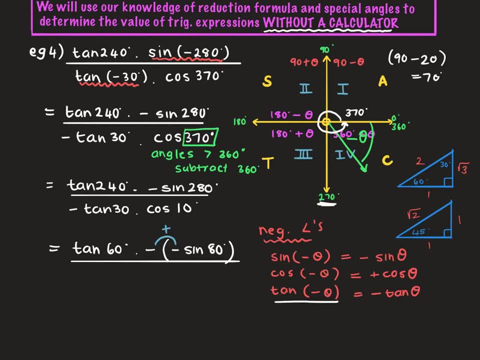 but I'm just going to keep using reduction formula, All right. So at the bottom we already have the acute angle, negative tan 30 and cos of 10.. The angle is also acute, So I don't need to simplify those any further. 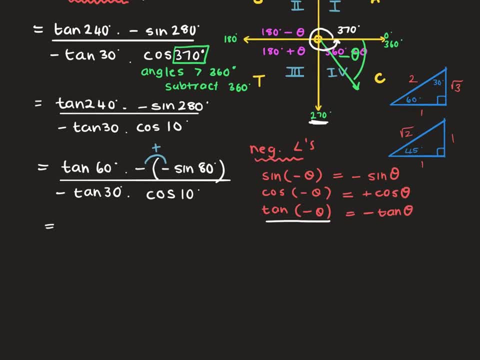 All right, let's wrap this up. Tan of 60.. All right, So tan of 60, opposite over adjacent. So tan of 60 is root three, All right Times, positive sine 80.. All right, So remember now that sine of 80 or 80 degrees. 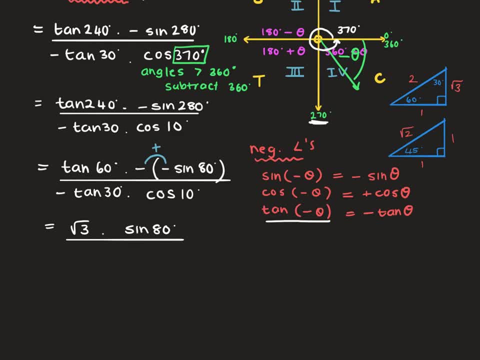 is not, from my special triangles, Correct, But I see this juicy: 10 degrees sitting in the denominator and 80 degrees in the numerator, And what do those add up to 90 degrees. So we're going to simplify those using our co functions. 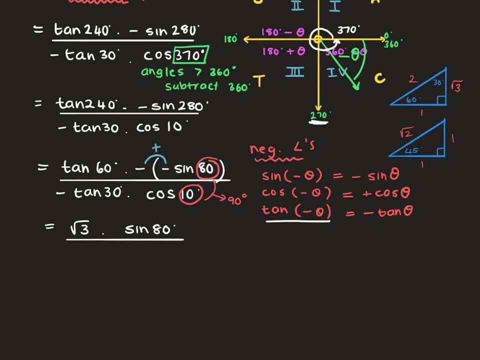 Okay, But let's not get ahead of ourselves. Um, we need to deal with negative tan 30 first. So tan of 30 opposite over adjacent. That's what we're going to do. So tan of 30 opposite over adjacent. 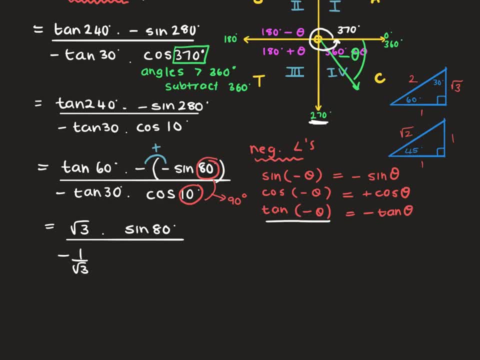 That's what we're going to do. So tan of 30, opposite over adjacent, That's going to be negative one over root three. So, like I said, this idea here with your co functions, I'm going to rewrite cos 10 as sine 80.. 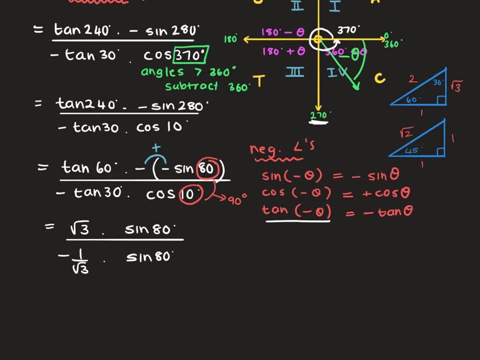 We know that those are equivalent in value. And if you want to check, punch it in on your calculator: type cos 10, type sine of 80. Okay, So now this is lovely because those can cancel. So now this is lovely because those can cancel out. and what's left over for 11th? 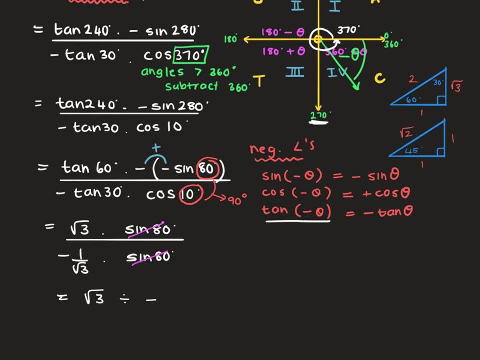 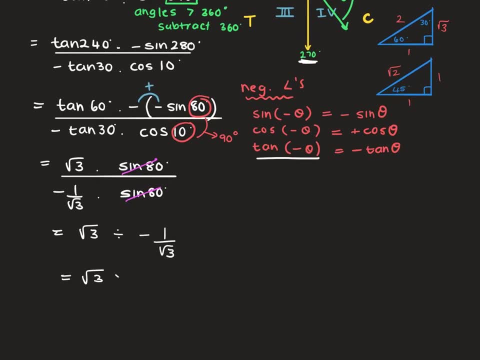 We have root three divided by negative one over root three. What does that become? That will be root three times negative root three over one, And we know that if we multiply those two surds together, your final answer is just going to be minus three.